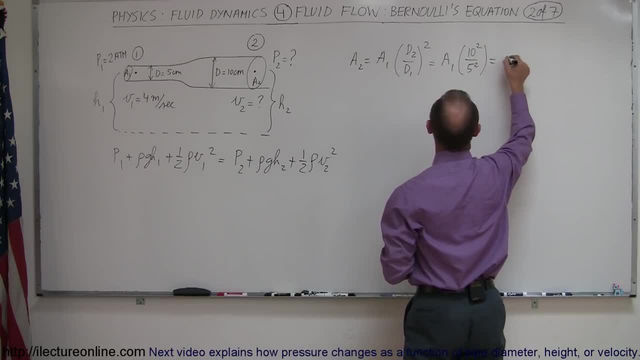 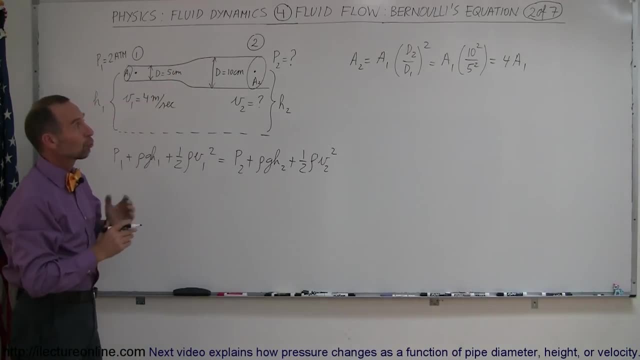 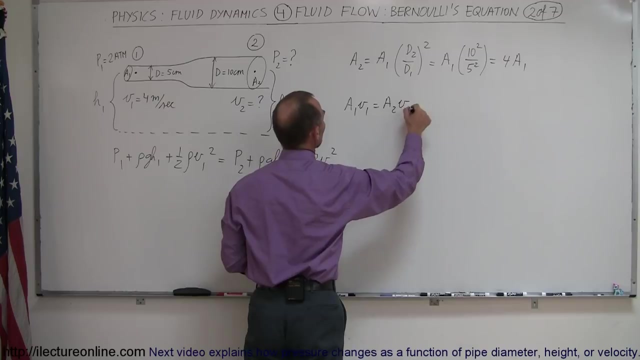 over 5 squared, that would be 100 over 25, or 4 times a1.. So we can see, by doubling the diameter of the pipe, we quadruple the cross-sectional area, and because we could say that a1, v1 is equal to a2, v2, that then implies that v2 is equal to v1. 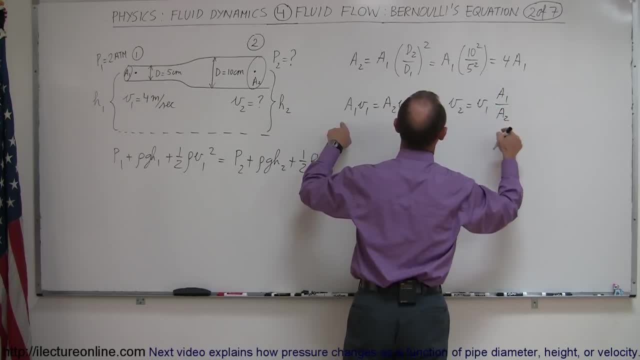 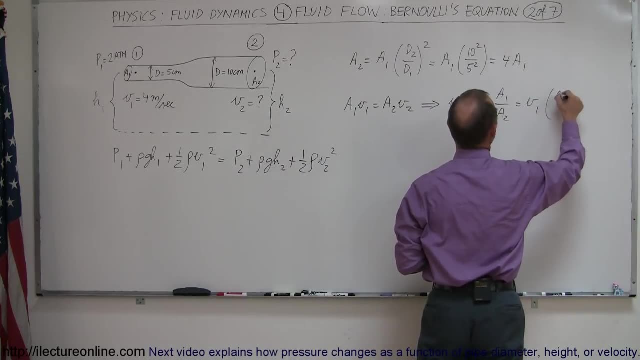 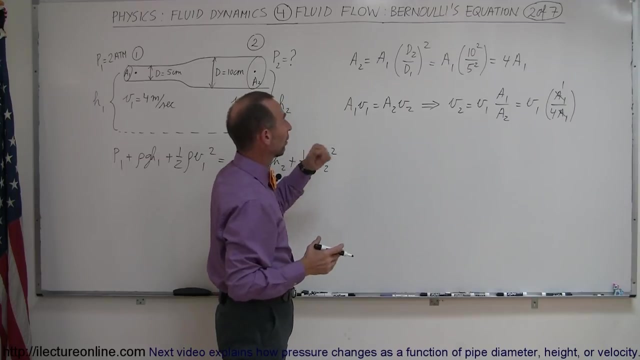 times a1 over a2.. Now, since a2 is four times as big as a1, so we could say this is equal to v1 times a1 divided by 4 times a1.. This cancels out, and so now we can see that v2 is one quarter of v1, so if v1 is four meters per second, 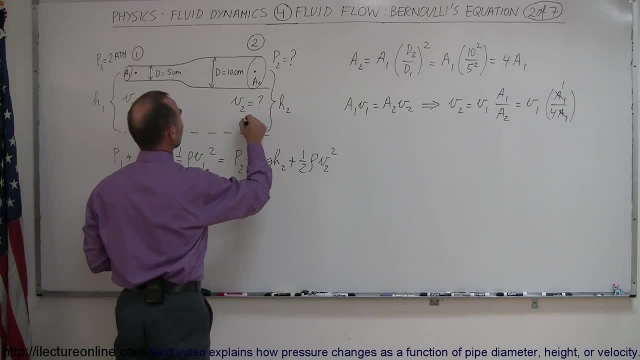 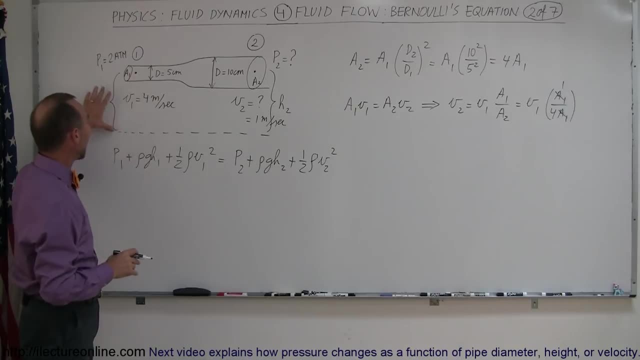 then v2 has to be one quarter that, or one meter per second. All right, so now that we know that, we're now ready to tackle Bernoulli's equation. First of all, the height doesn't change, which means that the term rho gh1 and the term rho gh2 has to be exactly the same. They stay constant. so 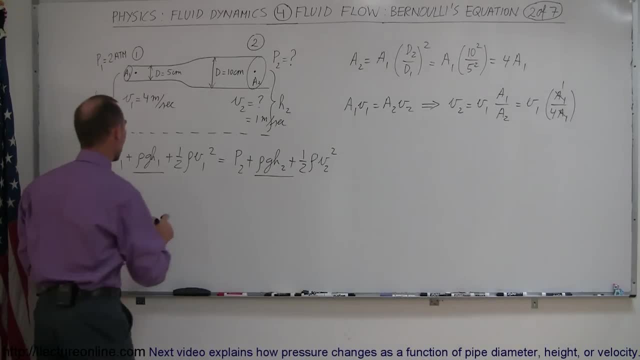 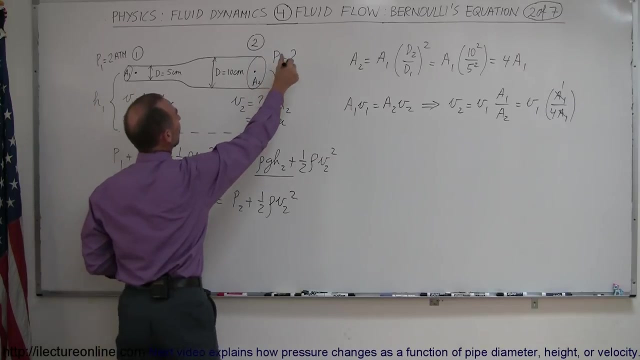 I can go ahead and divide or just simply remove it from both sides of the equation, which now means the equation then simplifies to: p1 plus one half rho v1 squared equals p2 plus one half rho v2 squared. So since I'm looking for p2, that's ultimately what I'm after right here. I can then solve: 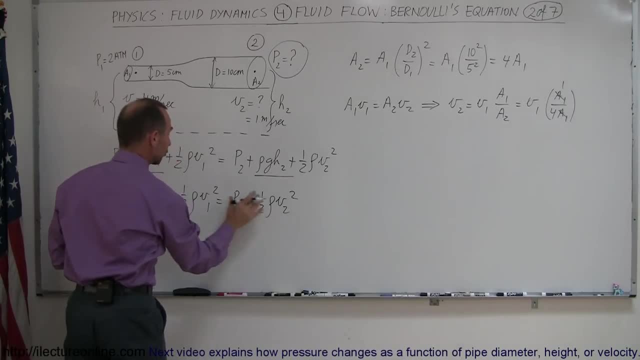 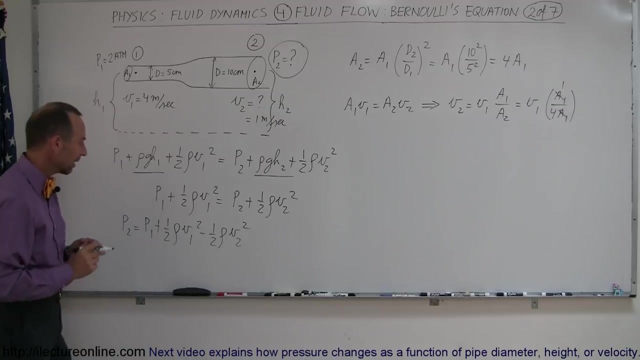 this equation for p2.. I can move the one half rho- v2 squared to the other side and flip the equation around. so now I end up with: p2 is equal to p1 plus one half rho- v1 squared, minus one half rho- v2 squared. All right, now I think I'm ready to. 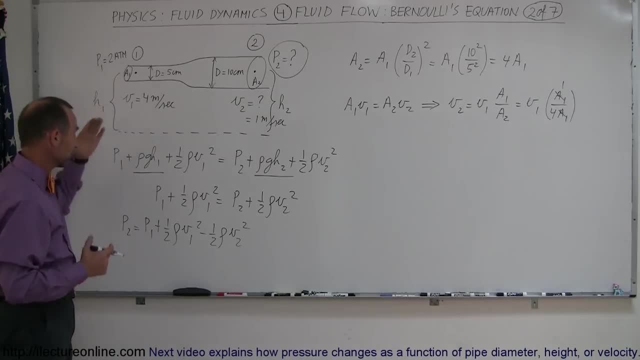 plug in some numbers. First of all, p1 was two atmospheres, so we can leave that there. or before I do that, you know what I think- I'll factor out a one half rho. that makes it a little bit easier. So p2 is equal to p1, plus one half times rho, times v1 squared minus v2 squared. That makes it a. 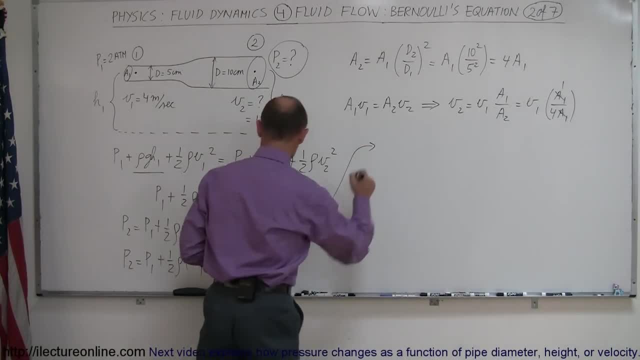 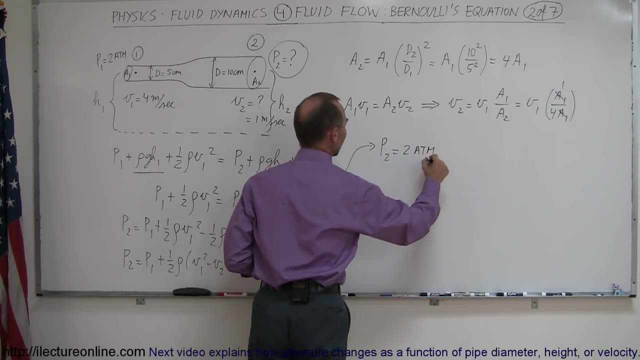 little bit easier to work with. Let's move over here. Plug in. p2 is equal to p1, which is two atmospheres. we don't have to convert that to pascals. that is fine, plus one half times the density. assuming that this is water, the density 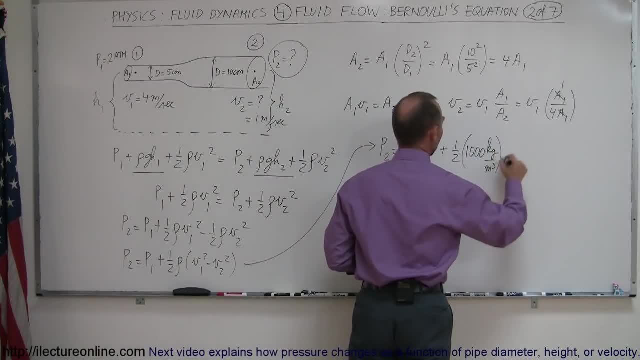 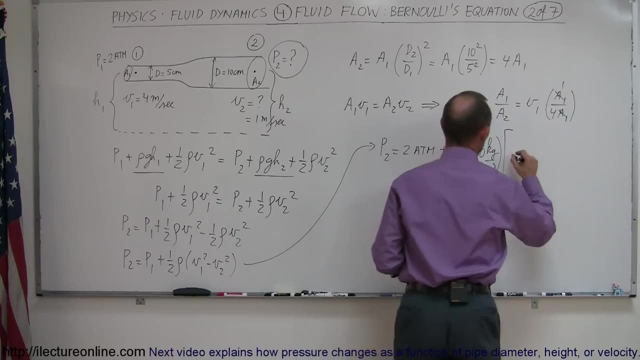 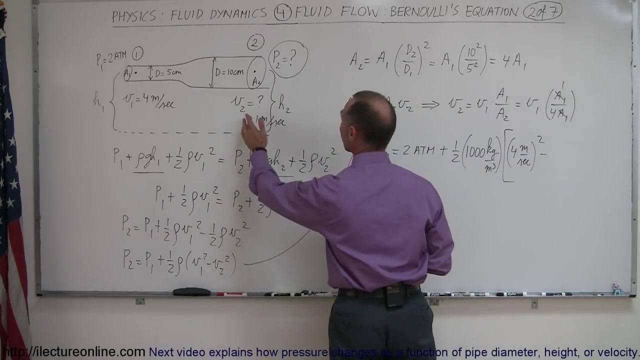 water is 1000 kilograms per cubic meter and then I multiply that times v1 squared minus v2 squared. Now, remember, v1 squared was four meters per second, so that's four meters per second. we have to square that minus v2, which was only one meter per second, so that's one meter per second, and we have to square. 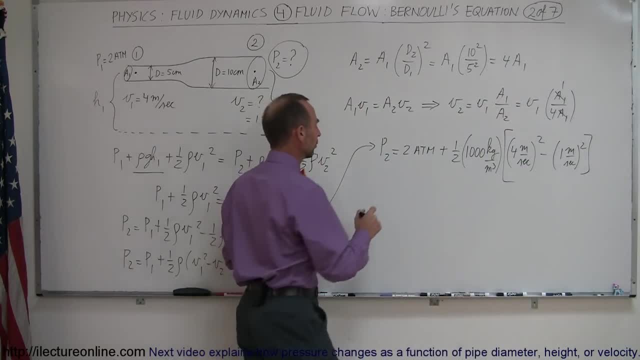 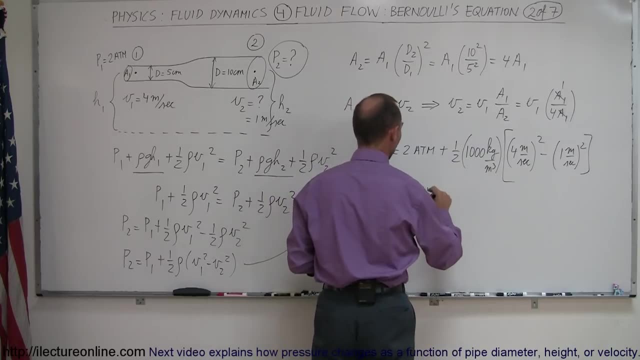 that. so it would be 16 minus 1 or 15. so we have: p2 is equal to two atmospheres. one half of thousand, that would be, plus 500 kilograms meters cubed. and multiply that times 16 minus 1 or 15, that would be. 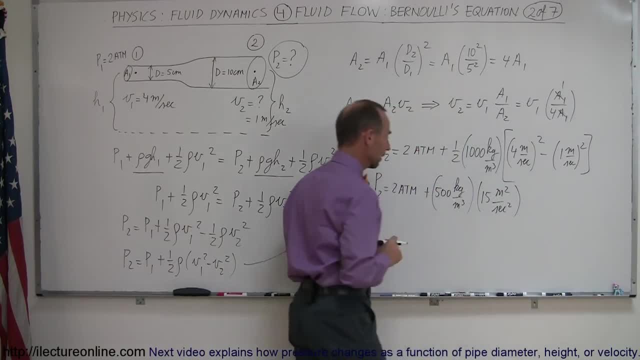 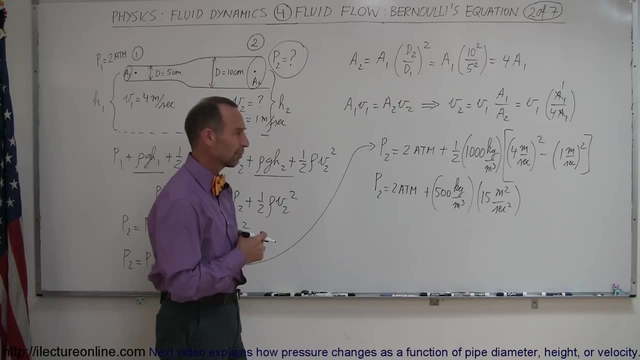 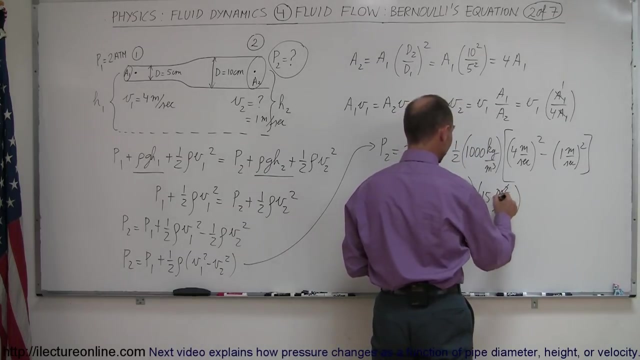 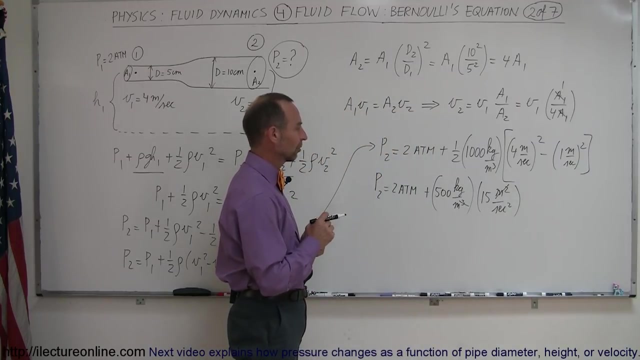 meters squared per second Square. all right, now, looking at the units, is kilograms per cubic meter times meter squared per second square. is that pascals? hmm, I don't know, let's find out. well, first of all, this cancels out with two of those. so now we have kilograms per meter per second square. but I need pascals, I need a unit of pressure. 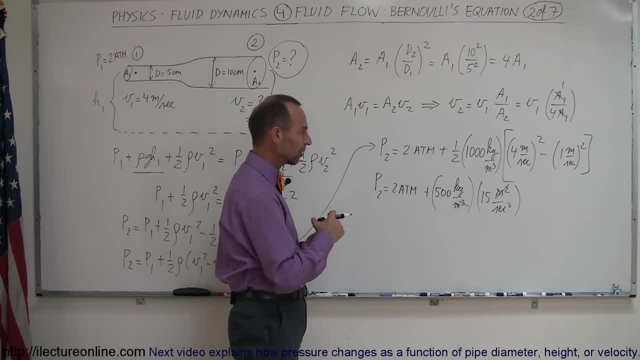 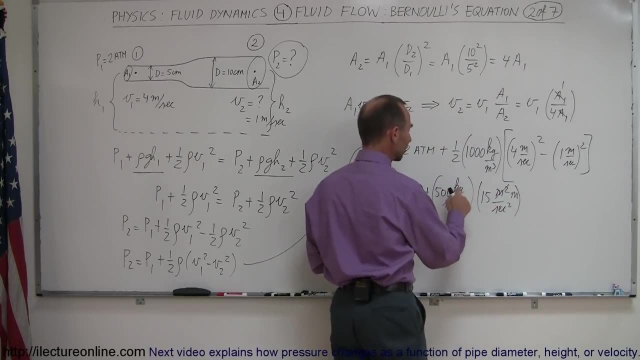 which is newtons per square meter, and a newton is a kilogram meters per second square. so it looks like I do need a meter here and I do need another meter over here. so that means kilograms meters per second square divided by meter square, which is indeed pascals. so units work out all right. so what's 10 times 15 times 500? so pressure two is equal to two atmospheres plus. hmm, that's interesting. 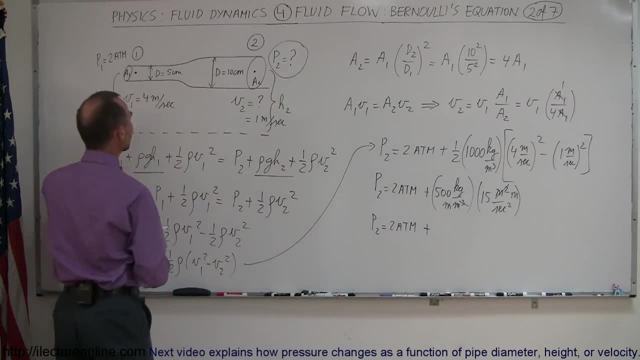 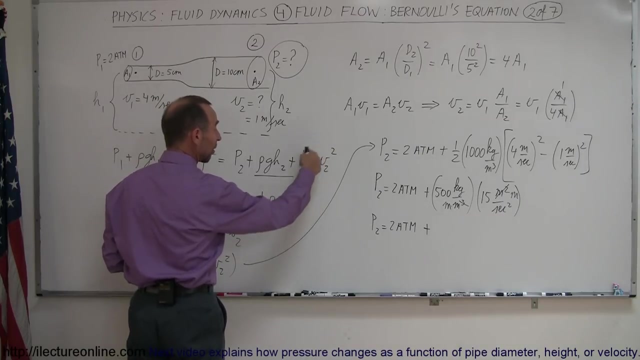 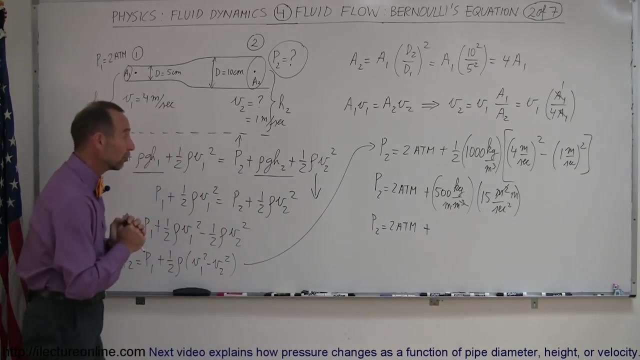 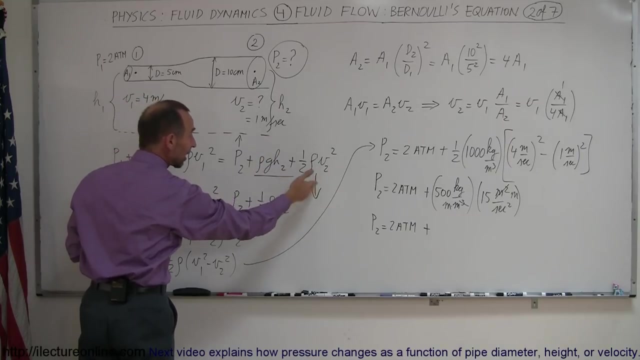 That's interesting. If the velocity slows down, it indicates that the pressure goes up. does that make sense? well, let's find out here. So here we have: if the velocity becomes smaller, well, if this becomes a smaller quantity, then something else has to get bigger. so this becomes smaller. that means this has to become bigger, which is indeed what we're finding. so with Bernoulli's equation we can see, first of all, when the height goes up, pressure goes down, but when the velocity goes down,